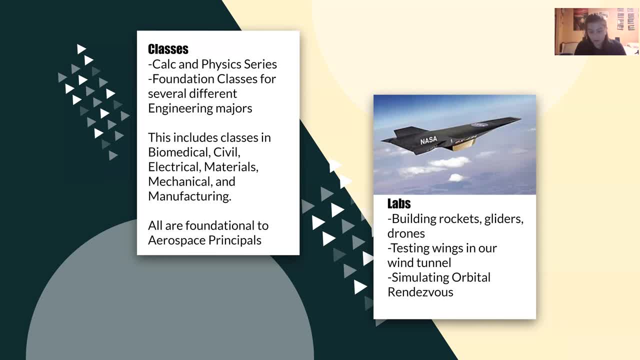 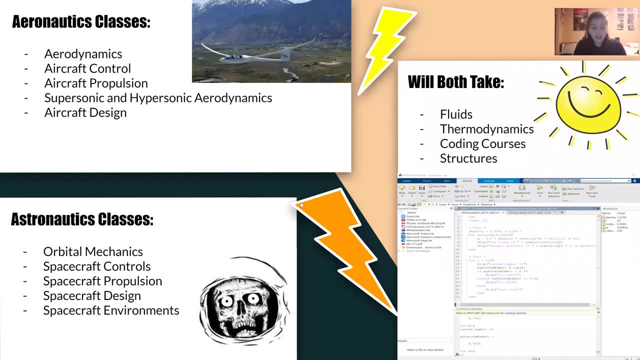 you get to take an intro aero class where you actually get to build your own rocket and glider and really get a feel for what both concentrations entail. You don't have to choose your concentration until your third year. If you choose air, you spend the next two years taking courses in aerodynamics. 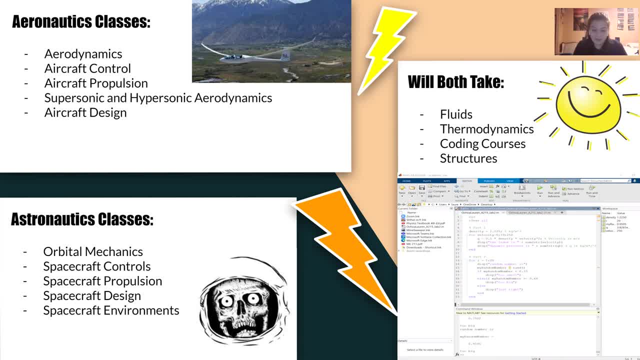 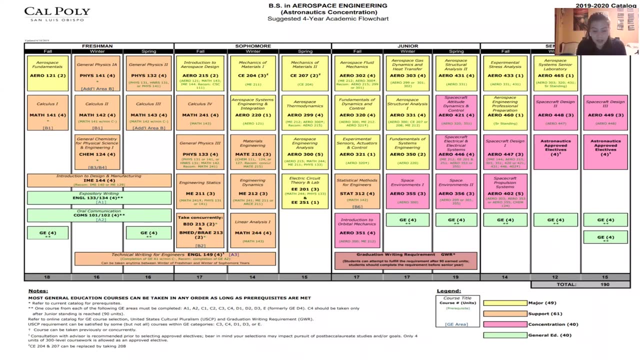 aircraft control and engineering. You don't have to choose your concentration until your third year. If you choose space, you spend the next two years taking classes in orbital mechanics, spacecraft propulsion, spacecraft design and spacecraft environment. I've included pictures of the flow charts for aeronautics and astronautics. 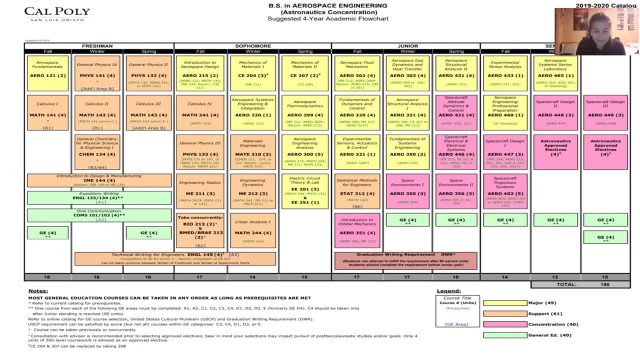 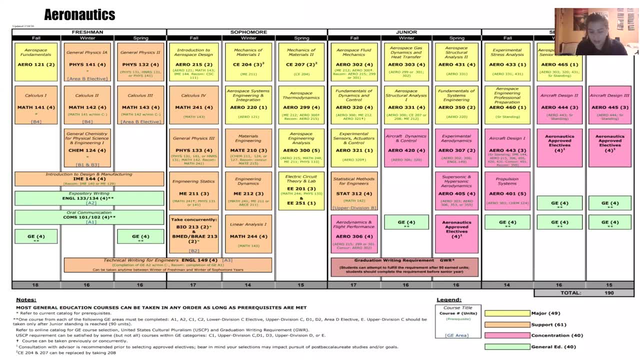 This one is astronautics. Of course you can deviate from the schedule quite a bit, especially the first two years, and especially if you come in with credits. Here's aeronautics. They're probably the most important thing in your life. They're the most important thing in your life. They're the most important thing in your life. 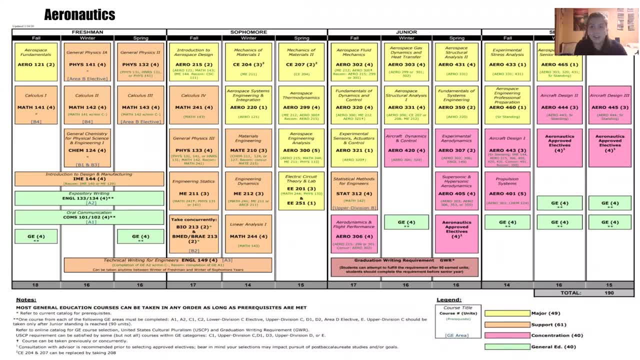 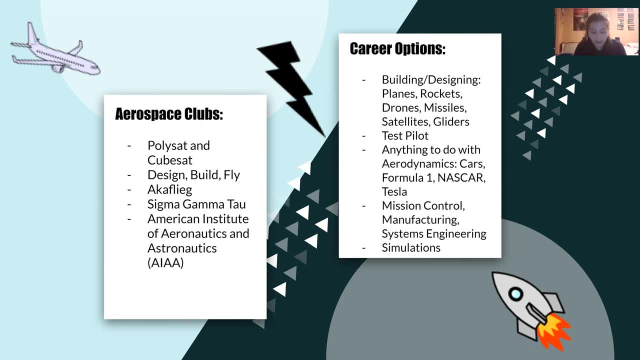 They're both basically the same, other than the concentration or pink courses. Now, if that's not enough for you, we also have a bunch of cool aerocentric clubs. PolySat makes their own little satellites and partnered with NASA and other companies. 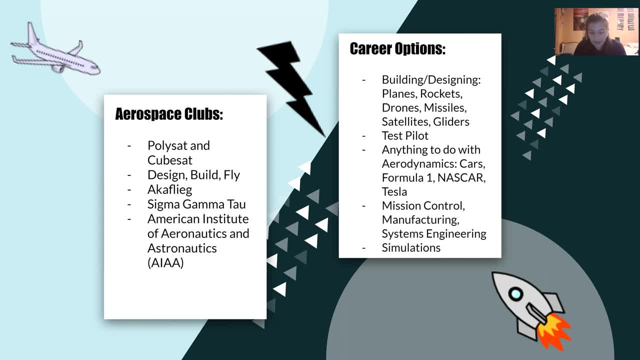 actually get to launch them into orbit. Design Build flies: designs and builds RC airplanes and flies them in AIAA competitions. Aquafleek is a club designed to help students get their glider license and work on glider- based projects. 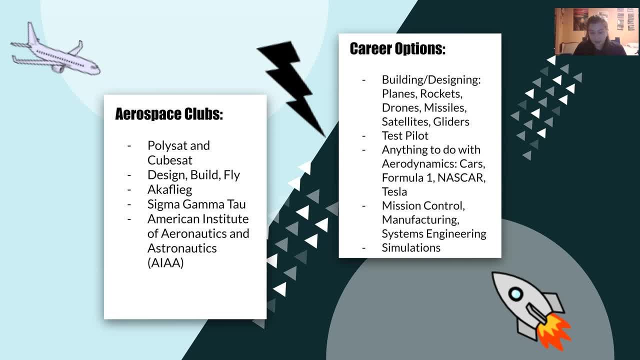 SIGMA Gammatale is an aerospace engineering honors society and AIAA is a professional club that helps students connect with industry. There's a lot you can do with an aerospace degree, especially since it's an ever-growing industry. Just to name some career options, you can help build and design planes, rockets, drones, missiles, satellites, gliders. 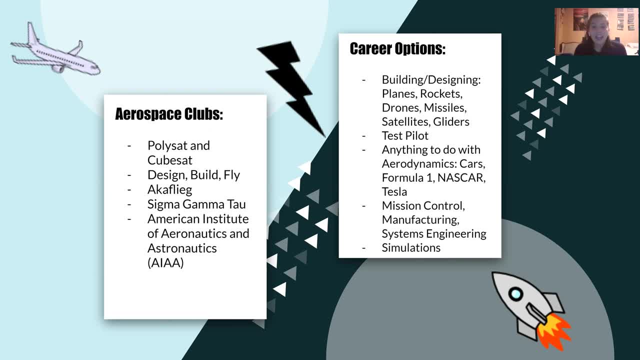 You could be a test pilot. You can work with simulations, Really anything that has to do with aerodynamics. so cars, companies like NASCAR and Tesla, If you're on the space side, you could work as mission control. or, if you want to be, on the 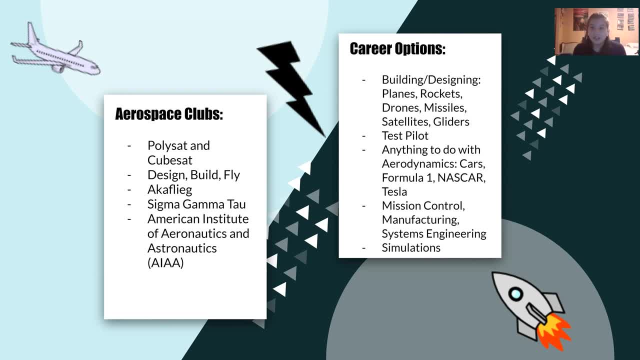 ground. you can be a manufacturing engineer, which actually builds the rocket and satellites, or you could be a systems engineer, which is more like the managerial position, making sure all the pieces come together. Now, that's all I have for my slideshow, so thank you so much for watching.